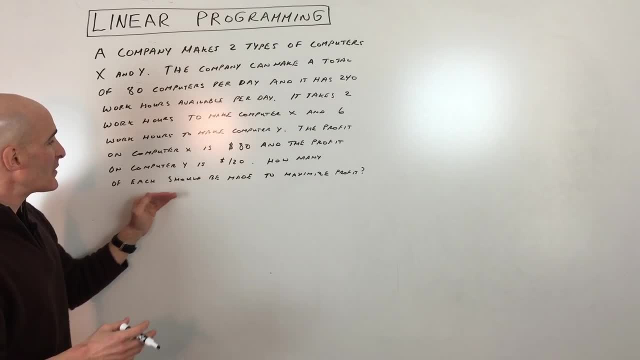 help to kind of frame the problem a little bit for us. So how many of each should be made to maximize profit? So let's see what's an equation for the profit. Well, profit equals $80 times the amount that's made on computer X. okay, plus $120, which is made on computer Y. 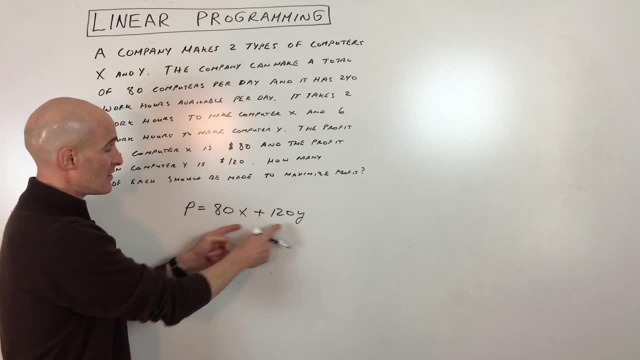 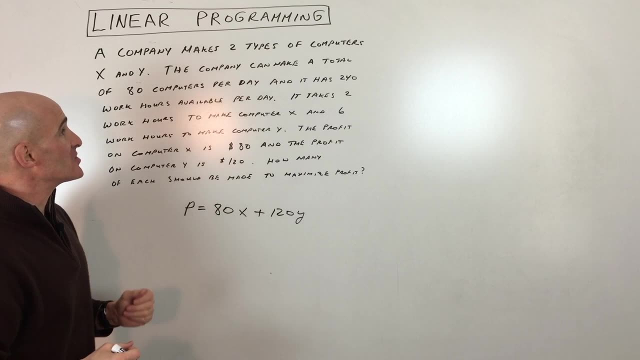 So if we can figure out how many of X and Y type computers we should make, that'll be the profit, right? Okay. now what we want to do is we want to work with the constraints. okay, the constrictions, the restrictions. right. So it says you can only make a total of 80 computers per day. Okay, 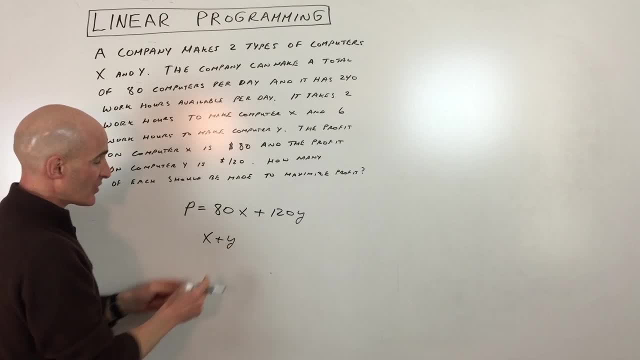 so what does that mean? It means that X plus Y- okay, the two types of computers- make less than or equal to 80, okay, right, Okay, what other restrictions are there? It only has 240 work hours available. Okay, so that means you can't work more than 240 work hours. It has to be. 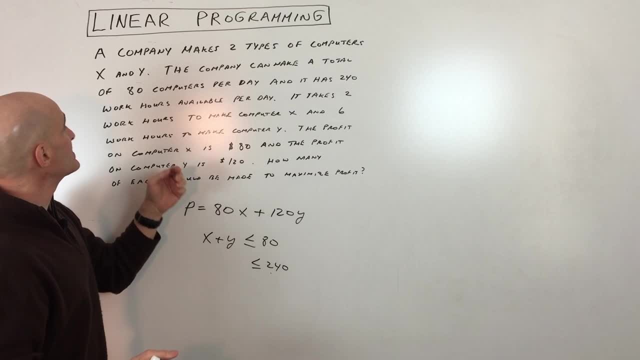 less than or equal to 240 work hours. And let's see: it takes two work hours to make computer X, so that's 2X. It takes six work hours to make computer Y, so that's 6Y is less than or equal. 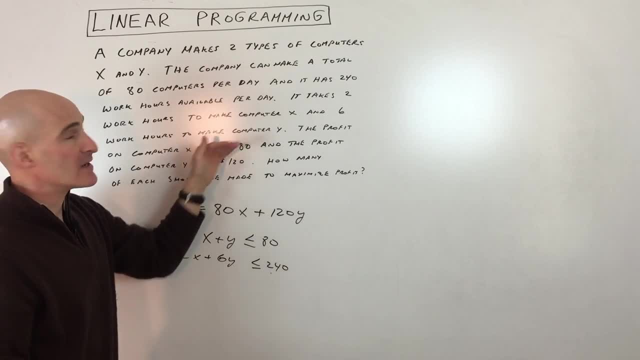 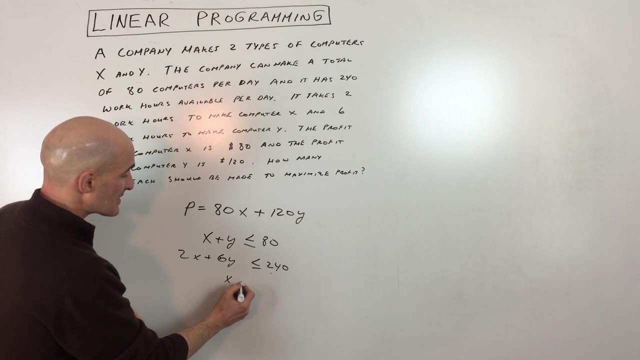 to 240.. Now, something that's not always written in the problem itself is the fact that you can't really make a negative number of computers. so we have to assume that X is greater than or equal to zero. Can't make a negative number of computers. right And same. 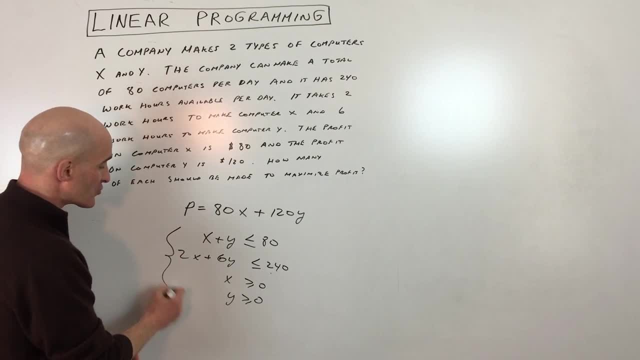 thing with Y: Y is greater than or equal to zero. So these are constraints, and what we're going to do is we're going to graph this now and we're going to look at the region- okay, the feasible region that satisfies all these constraints. So let's go ahead and do that right now. Let's go. 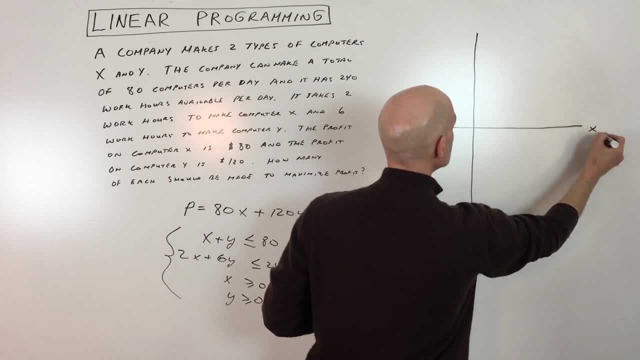 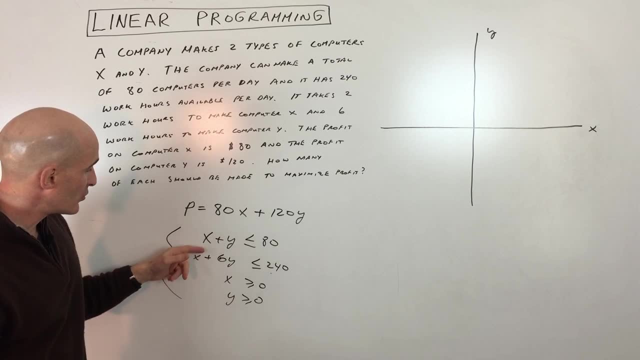 ahead and graph that. Okay. so what we have here is here's X, here's Y. Now what you want to do when you graph these is you want to kind of pay attention to, maybe, what the X intercepts and Y intercepts are. So it looks like here you're going to look at 80.. It looks like here it could be like. 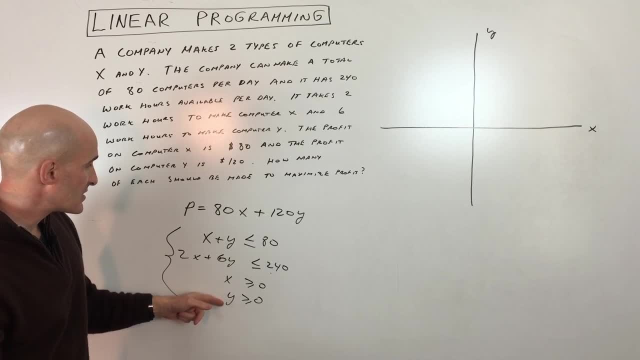 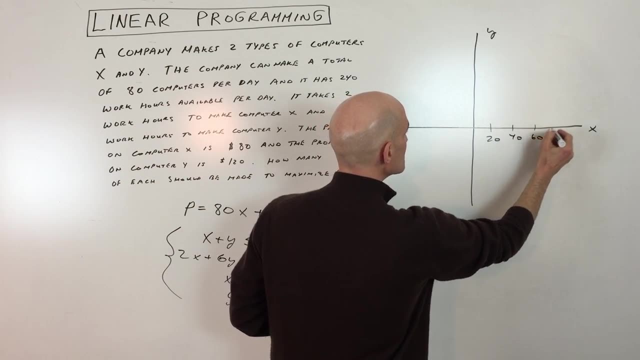 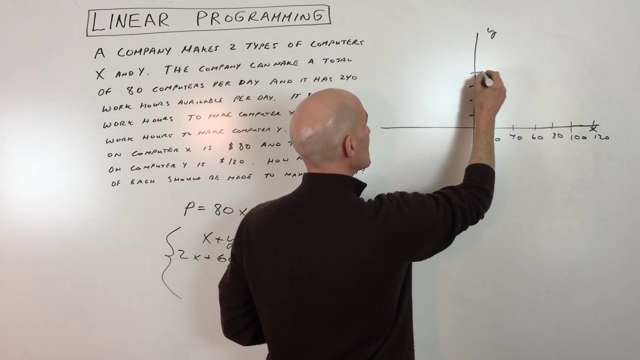 maybe 40 and 120, and let's see. So it looks like maybe we should count by like 20s. All right, let's do that. So we've got 20, 40, 60, 80,, 100, 120.. Same thing here: 20, 40, 60, 80, 100, 120. 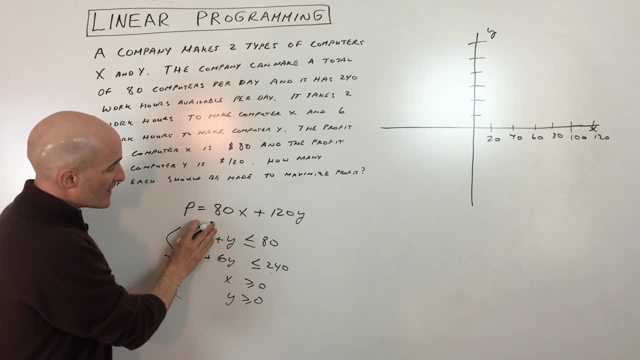 Okay, so now what I'm going to do is I'm just going to set X to zero, so Y is 80.. Okay, so 20,, 40,, 60,, 80, right there, And let's see if Y is zero. 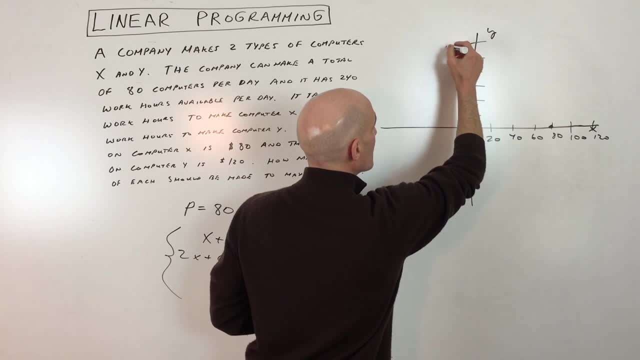 then X is 80.. Okay, good, And so if we graph our line, it's going to look something like this: And this is an inequality: You see how it's less than or equal to 80.. If we do a test point like 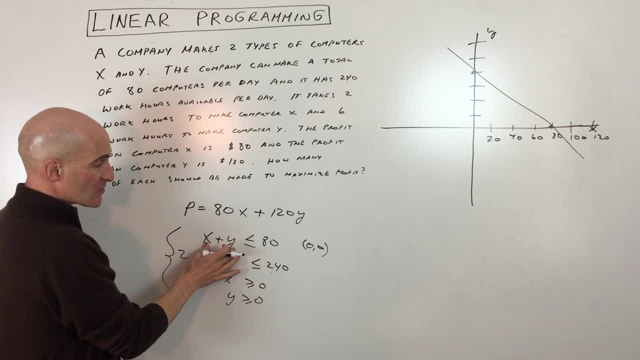 zero, zero. so we put zero in for X and zero for Y, So zero is going to be less than or equal to 80. So that means that where this point is here, that's the true region. So we want to shade in. 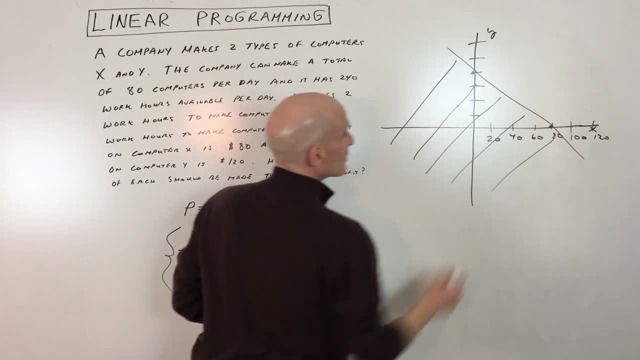 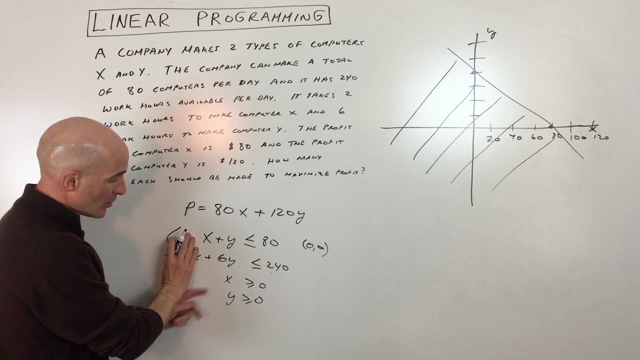 this region right here. Okay, All right. Now the next one. it says two X plus six, Y is less than or equal to 240.. So if we set X to zero, zero times anything is zero. divide by six, you can see our Y intercept is going to be. 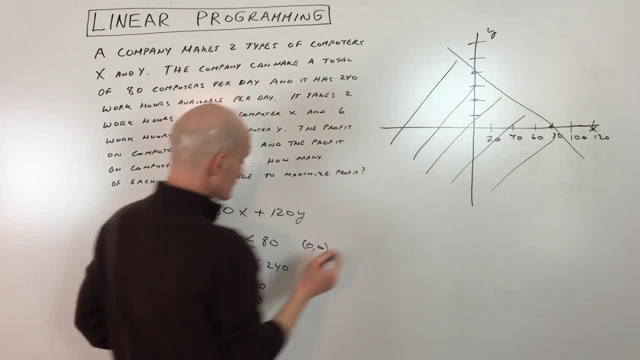 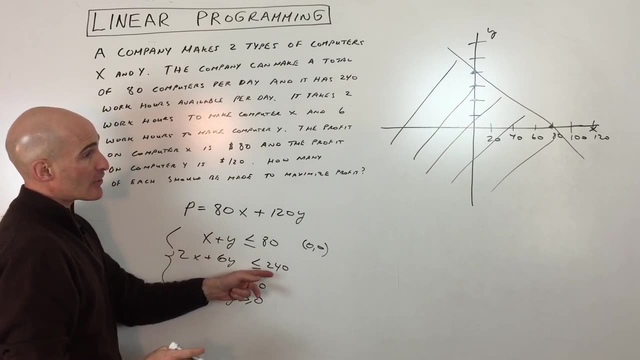 40. So that's 20, 40. So that's right there. If we set Y to zero, zero times six is zero, So that's why I'm covering that up. So then if we divide by two, you can see X is going to be 120.. So that's. 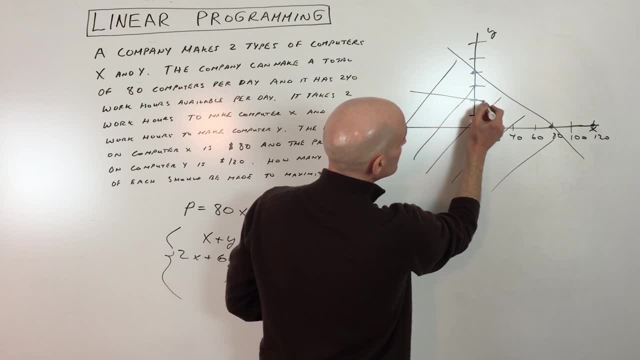 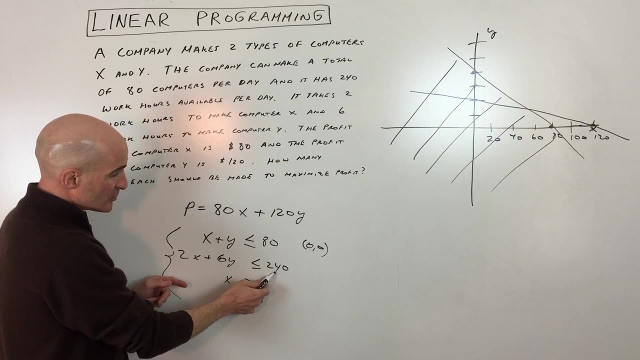 going to put us right over here And if we draw that line, it looks something like that, right. And again we do a test point like zero, zero is zero less than or equal to 240.. Yes, that's true. So that. 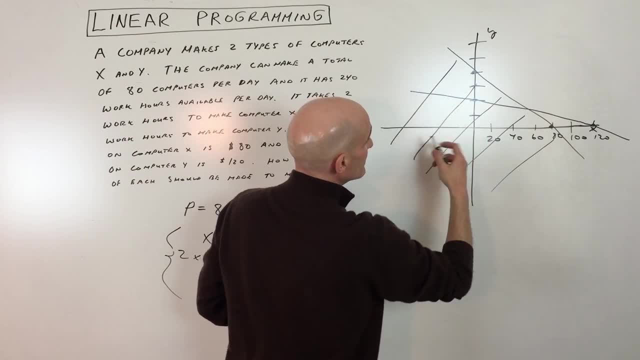 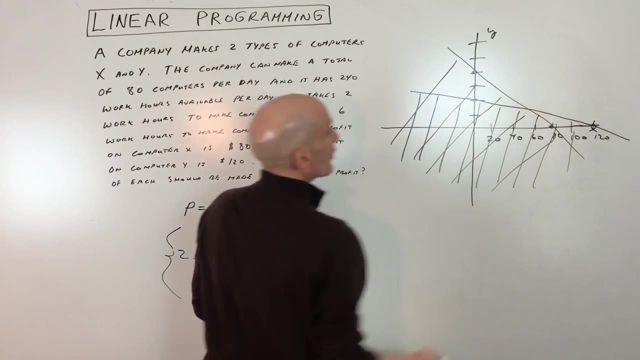 means that where this test point is, the origin is going to be on the true side of the line. So we're going to. that's going to put us right here, Okay, Okay. So so far you can see that we're. 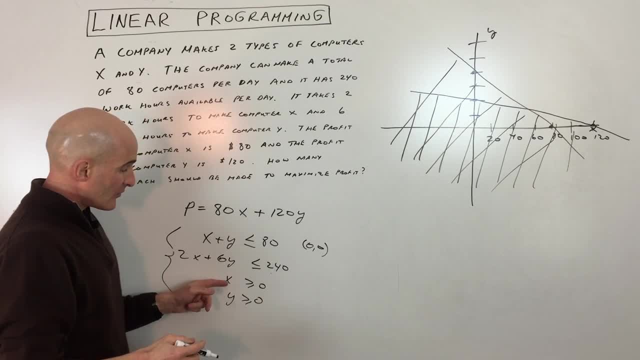 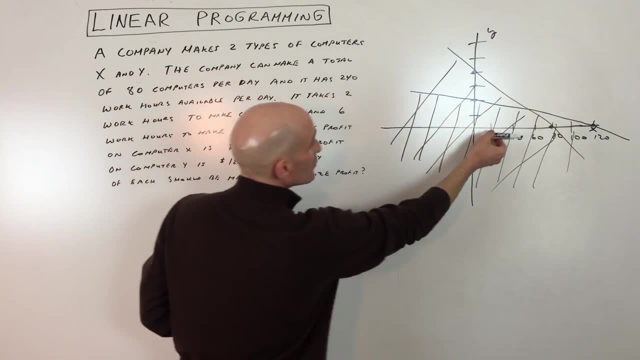 in this overlapping region. Now we also have to take into account that X is greater than or equal to zero. Okay, So that means we're to the right of the Y axis and Y has to be greater than or equal to zero, which means we're above the Y axis. 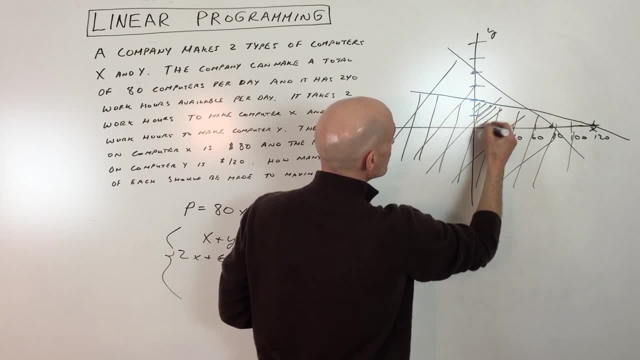 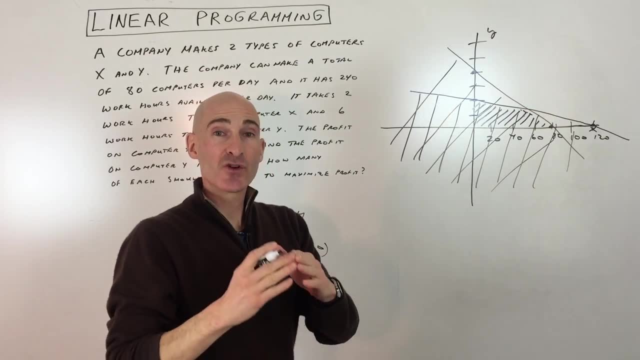 So you can see that all these regions, all these inequalities are overlapping right here in the first quadrant. Okay, Now the next thing you want to do is you want to look at the vertices or the corners of this polygon that's formed this region, And you can see there's a 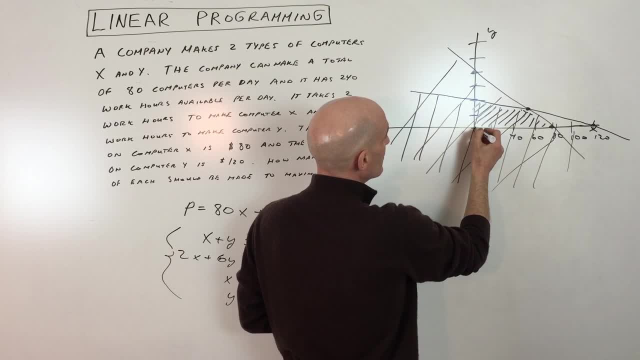 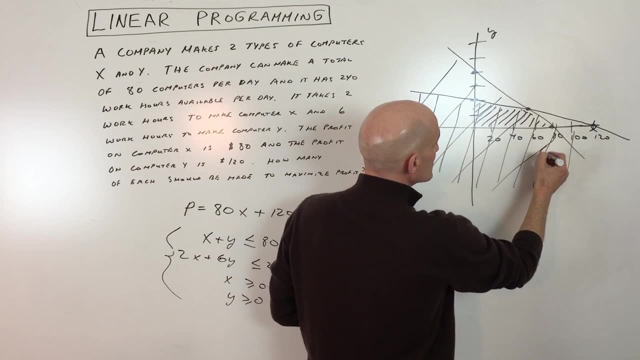 point here there's a corner, there's a vertex, there there's the origin and there's there. So what we want to do is we want to find the location of these points. Some of these we already know, like this point here is a 80 comma zero. This point here is zero comma. 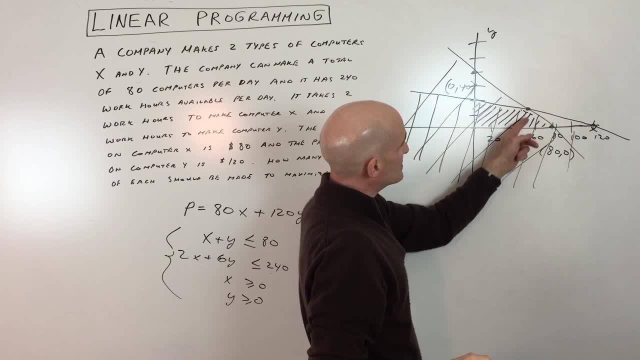 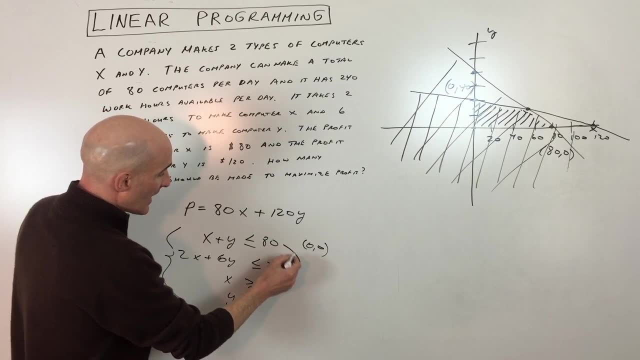 40,, right, But this point here is not so easy to to locate. Okay, It might be 60,, 20, but what we'll have to do is we'll have to take the two equations here of those lines, just treat them. 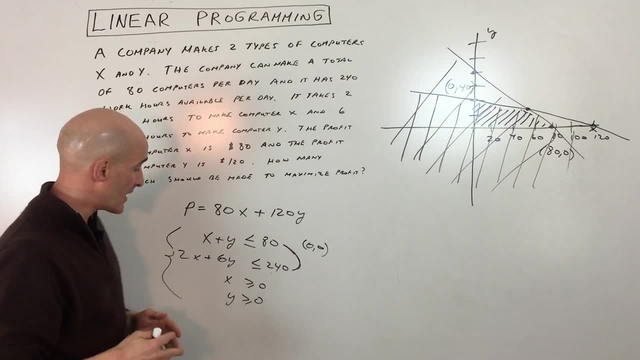 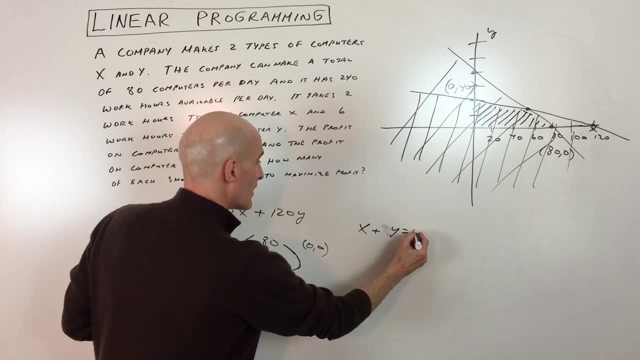 like equations And we'll have to solve that system to find out where they intersect. So let's go ahead and do that right now. I'm just going to write those over here and I'm just going to treat them like equations. So we have X plus Y equals 80, right. And we've got two X plus six Y equals. 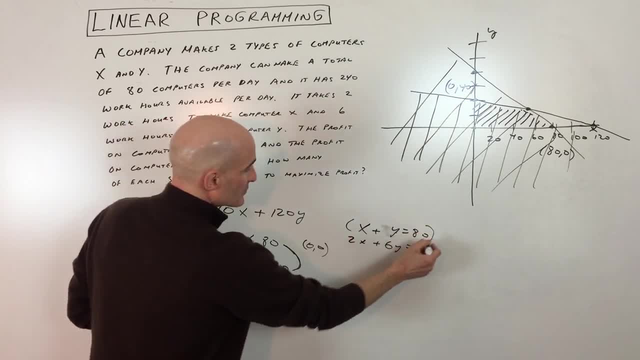 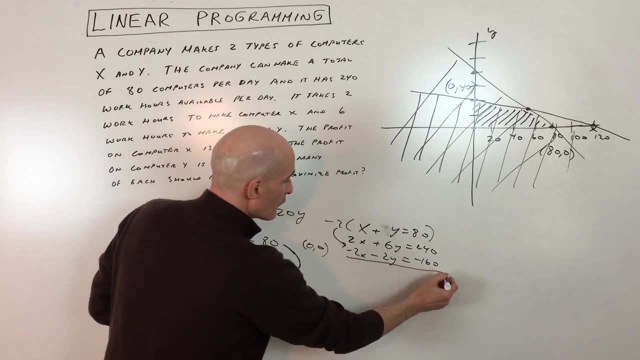 two, 40.. Now I'm going to multiply this top equation by negative. So I'm going to multiply this top equation by negative two, Okay, And I'm going to write it down here. So that's negative. two X minus two Y equals negative one, 60. If we add these together, we get four Y equals 80, right, So that. 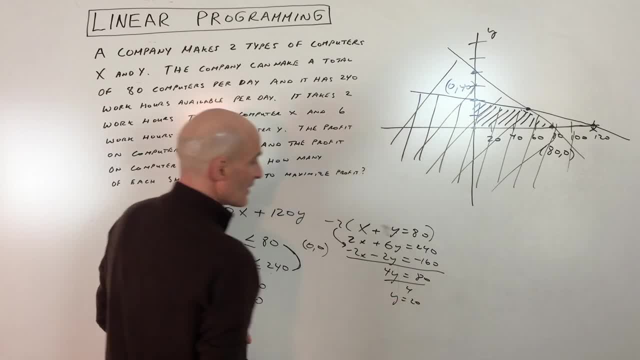 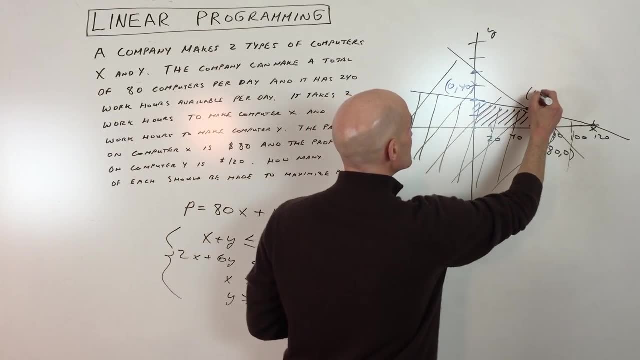 means that if we divide by four, Y equals 20.. And if we put 20 back in for Y here, you can see that X is going to be 60.. All right, So it looks like this point here is going to be 60 comma 20.. All. 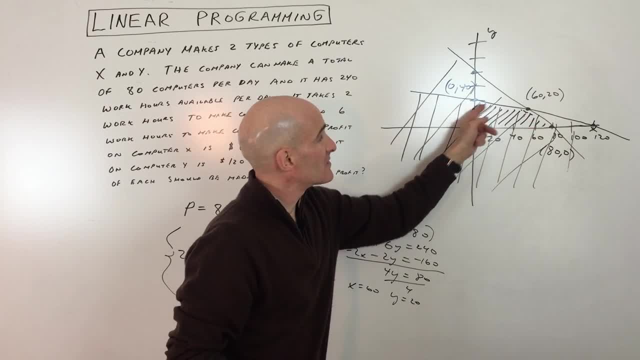 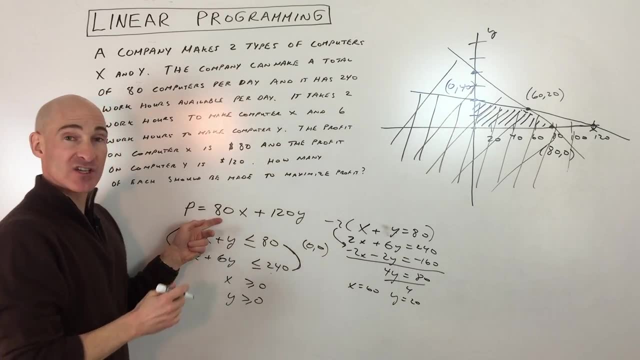 right. So now we've got the vertices, or the corners, of this feasible region. Okay, This polygon here that's formed the overlapping inequalities, And we want to test these in our profit equation, because we're trying to maximize profit. Now, sometimes you're trying to minimize. 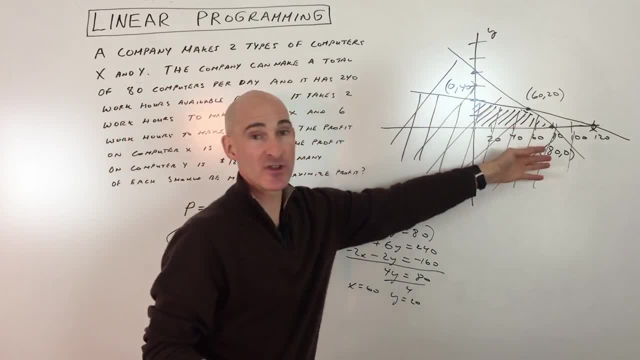 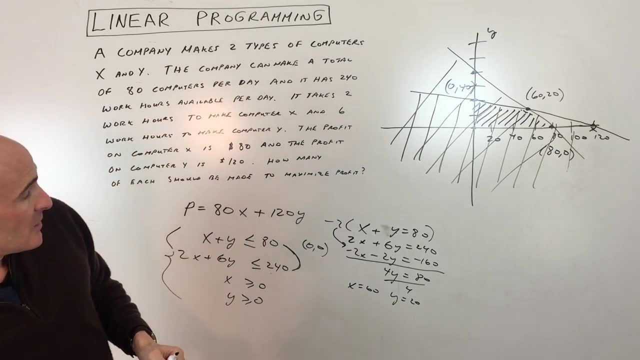 something like cost, and then you would plug in these points and see which is going to give you the minimum. but here we're trying to maximize, So let's go ahead and plug in zero, 40. So I put in zero for X and 40 for Y. What does that come out to? Well, we have 120 times 40, 4,800.. So at 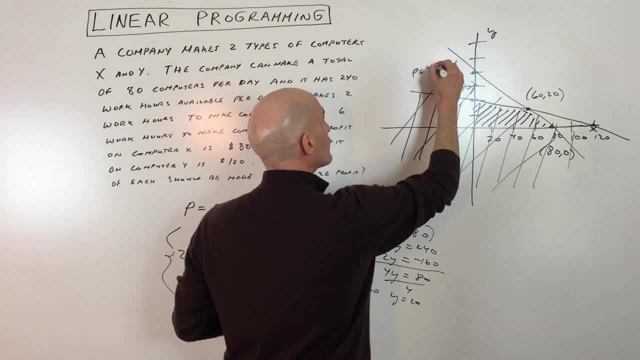 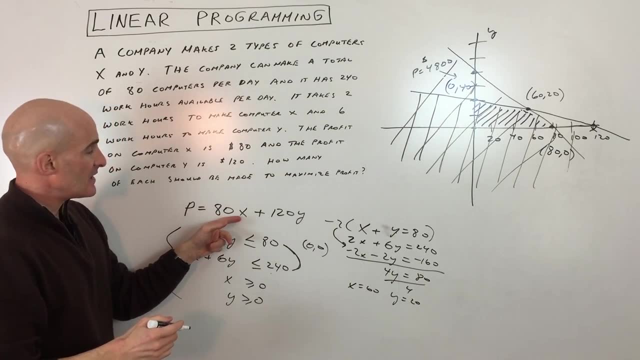 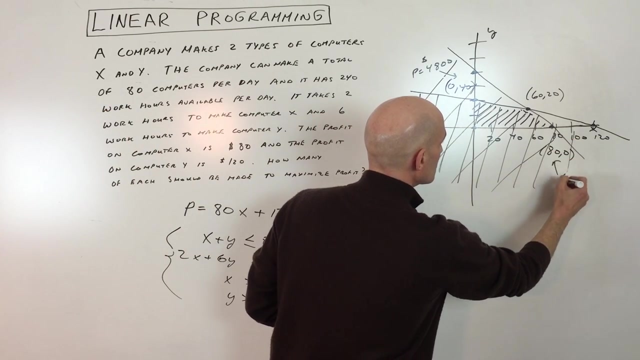 this point I'm just going to write: profit equals 4,800.. Okay, That's for this point, right here. Now let's go over to 80, zero. So 80, zero would be 80 times 80, which is what? 6,400 plus zero. So this point is going to be 6,400.. Okay, And then we're going. 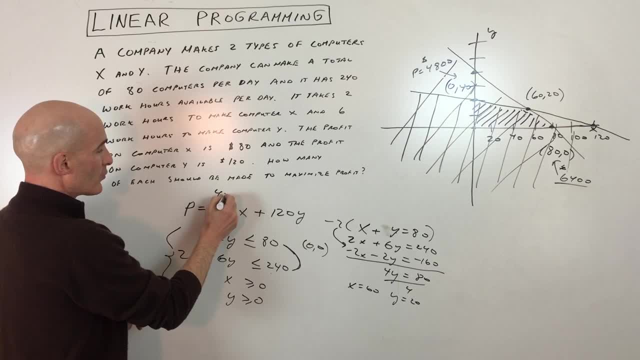 to check the 60, 20 points. So 60 times 80 is what? 4,800 plus 20.. That's going to be 2,400, right? So that's going to give us a total of how much. 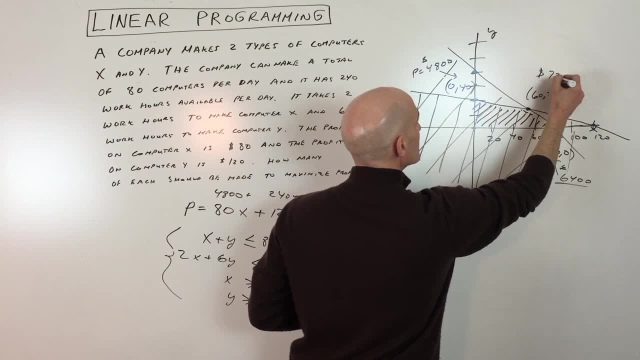 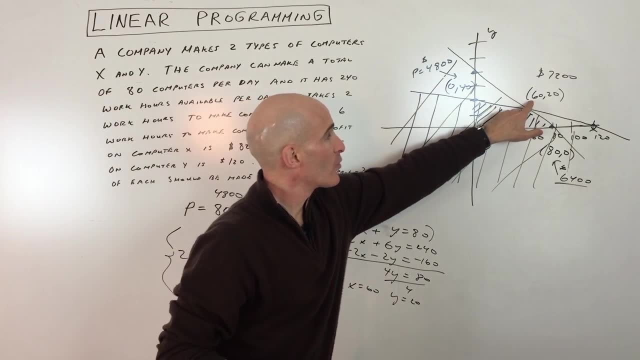 7,200, right, So this point is 7,200.. So it looks like if we want to maximize our profit here and still stay within our restrictions or our constraints, we're going to want to produce 60 of computer X and 20 computer Ys, right, And that's going to give you a maximum profit of. 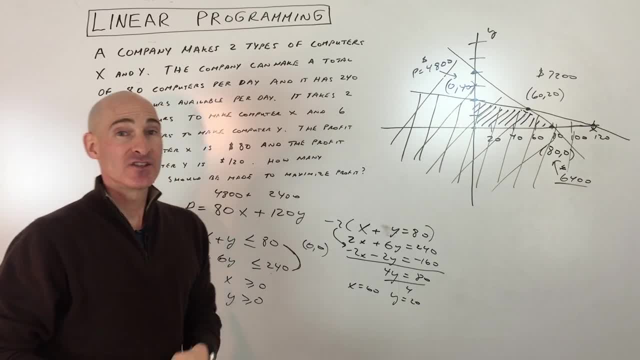 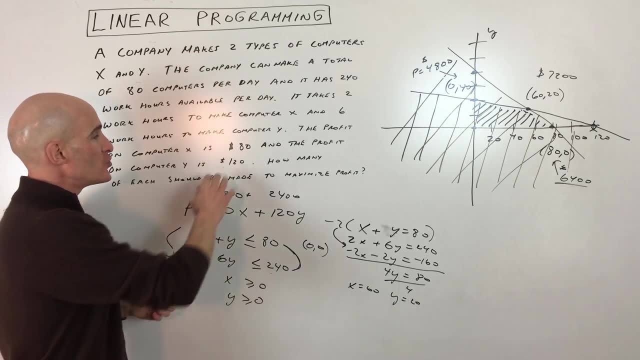 7,200. And again staying within the constraints. So a lot of work involved with these linear programming problems, but I think the key in my opinion is to just read it through quickly, That last sentence, trying to figure out what you're trying to maximize or minimize. Write that. 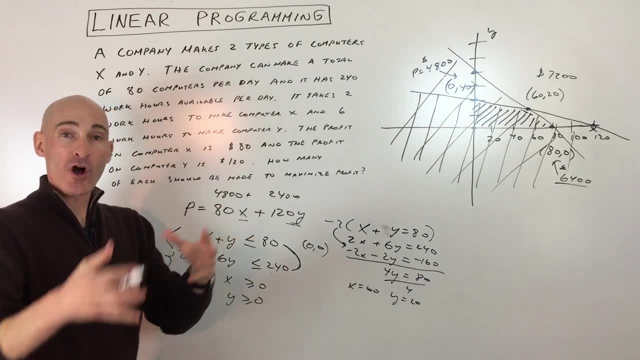 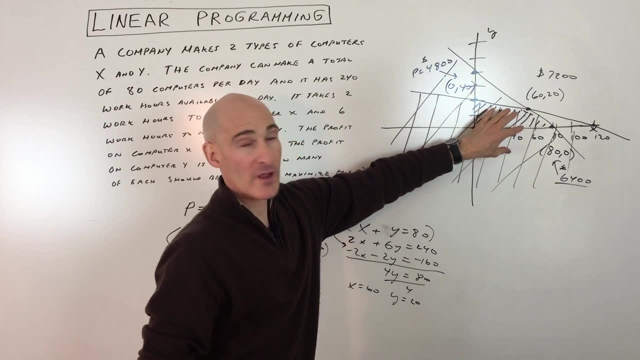 equation first. That'll tell you what your variables are. Then you can write all your other constraint equations in terms of those. you know those variables. Then go ahead and graph the region, Okay, Find out the overlapping region, And then what you want to do is look at the vertices. 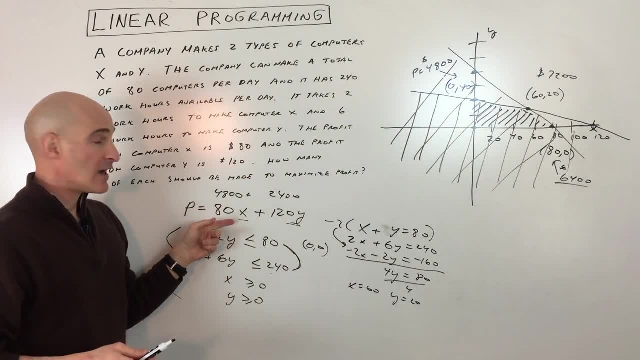 or the corners. Those are the points that you're going to want to test in your function, that you're trying to maximize or minimize- In this case, it was profit- And then whichever one gives you the largest or the least, depending on what you're trying to do, that's going to be what you're. 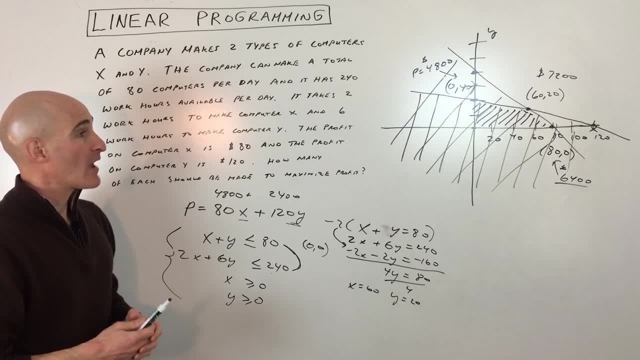 going to want to increase or decrease, So that's going to be what you're going to want to increase, So, and that's going to be your solution. So I hope this helped you understand how to work with linear programming problems better. Subscribe to the channel. Check out more math tutoring videos. 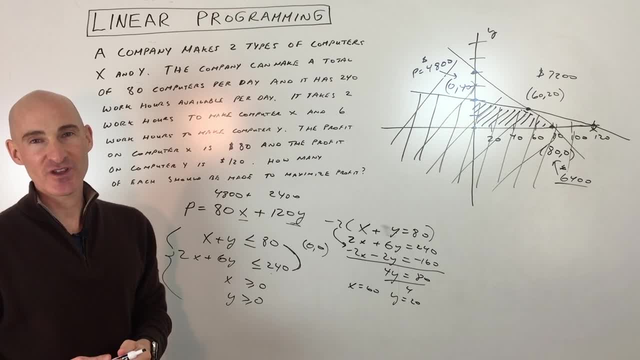 on my YouTube channel, Myra's Math Tutoring, and I look forward to helping you in the future videos. I'll talk to you soon. 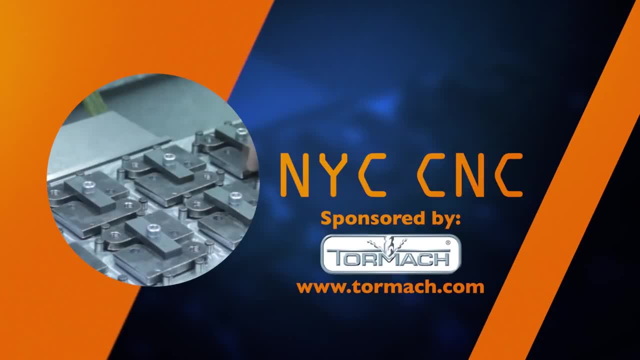 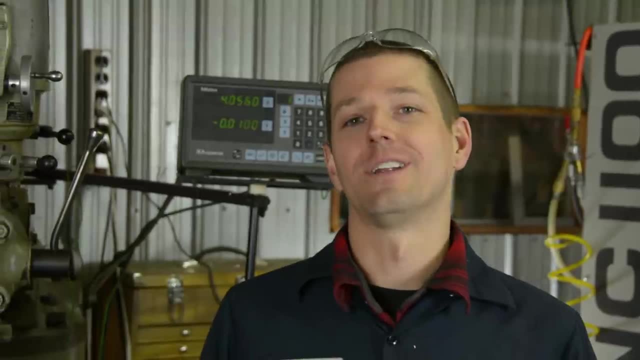 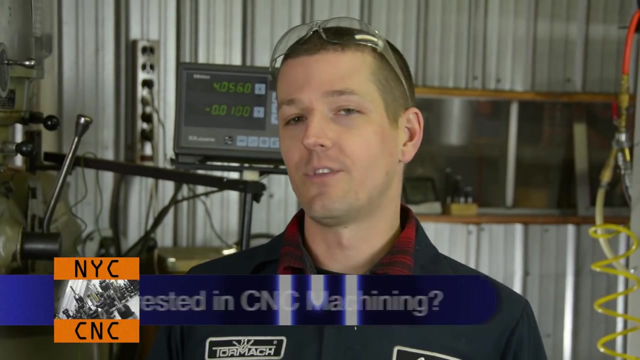 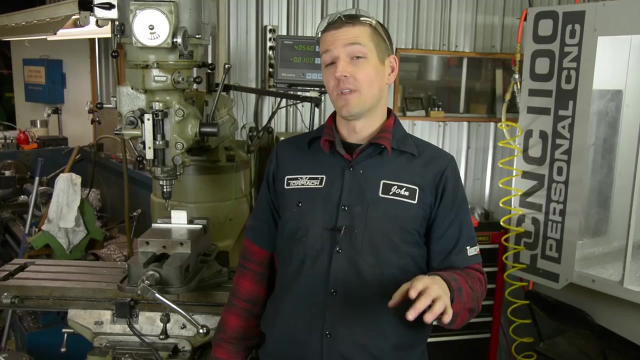 Hi folks, welcome to another episode of NYC CNC. This video is for the Concord Kids. They're a group of students that are focused on the STEM curriculum, and their advisor shot me an email and said some of the stuff that they're working on. it would be really helpful if they had a video that would show them some of the basics of what a milling machine does. And this really struck a nerve with me because, coincidentally, I was just talking to a local Ohio student.